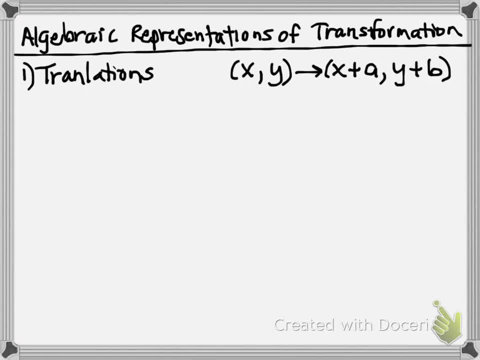 Faith. you're supposed to be writing this down, please, Okay, What I don't get to do when I finish, what I'm supposed to do is talk to people waiting for the next thing to be written down, Thank you. So if you have a positive a, 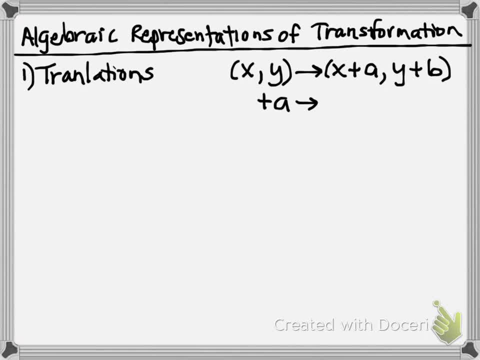 what direction does it tell you to move your shape. It tells you to move it right. So you're going to move right, a places, And again a represents some number. If it says minus a, what direction are you moving Left? 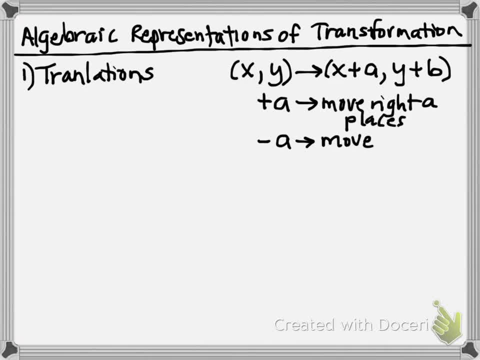 So the sign and the number are. We have to look at both of them. And again, a, And I'll put a in a quotation In a quotation Places. Okay, If you have a positive b, what direction are you moving? 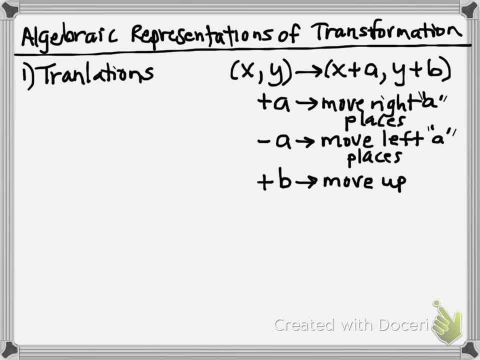 Okay, you're going to move up b places, And if you have a negative b, how are you going to move? If you have a negative b, you're going to move down B places. So sometimes they just make you do one. 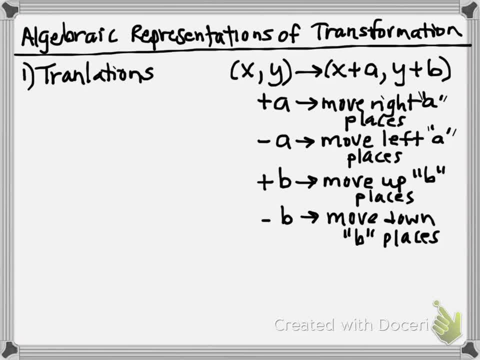 Sometimes they make you do both. Okay, So those are translations. So again you'll see numbers written in there, And when you are giving me the answer, if somebody says name the transformation, you can't just. Can you please excuse this interruption? 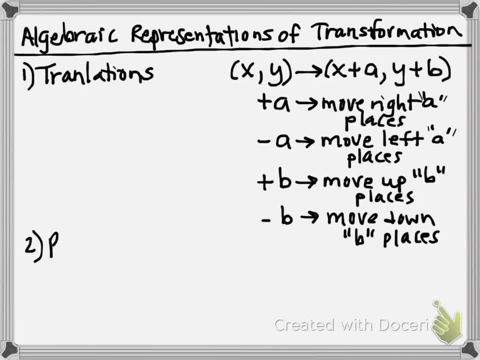 The next transformation. The next transformation is a reflection, And we have two different possible reflections. Actually, there's more than two, but the two that we're going to focus in on. All right, So the two type of reflections that we're focusing in on is one that's over the x-axis would be the first one. 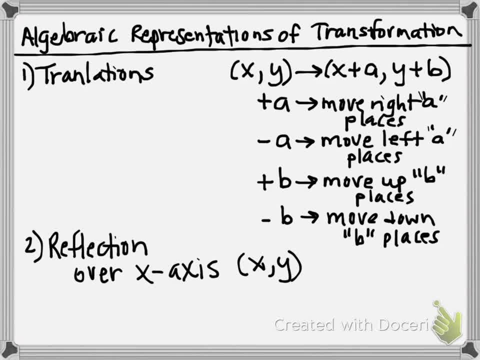 And the best way to remember what to do. The best way to remember what to do on this one is: look at if I'm reflecting over the x-axis. the x isn't going to change, It's the y that's going to change. 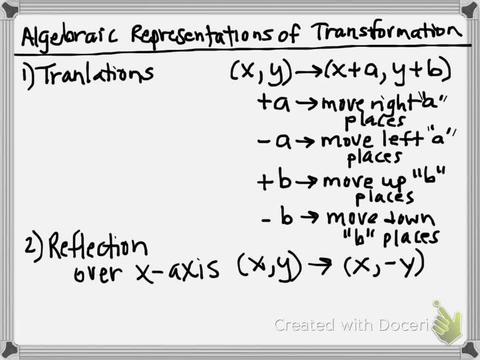 So we just have a sign change on our y's. Kenny, you need to write this, buddy. The other one is over the y-axis. So again, I would take my original ordered pair, And this time I'm going to have to change the x. 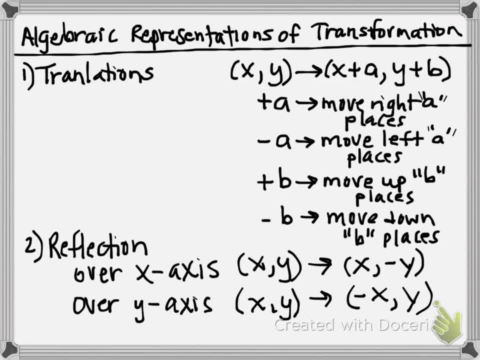 And I'm going to keep the y. And again, if you just take a picture and you're looking at, here's my shape and I'm going to reflect it over the x-axis. you're going to be in a new y value. 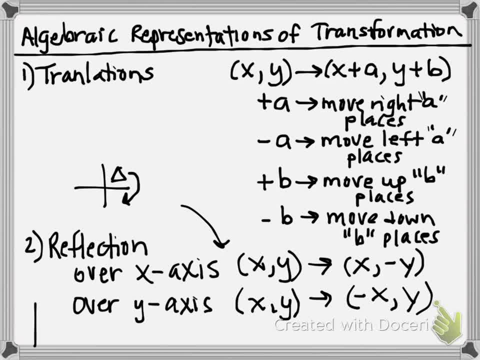 And so that kind of goes with this picture. And then if we do one here and we're going to go over the y-axis, we're going to go over here. So it makes sense that the x's now have changed signs. It'll come back. 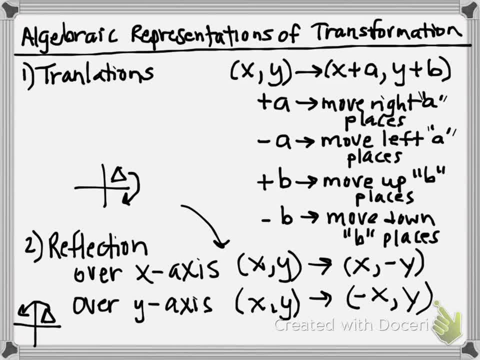 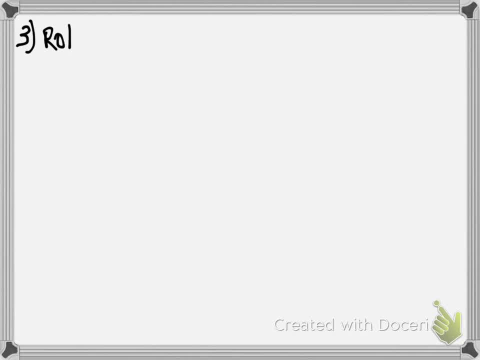 Okay, So the next one is the rotations, And that's the one that really, I think these algebraic representations help the best, And there's only three rotations that you guys actually need to focus in on. So with rotations, there is a 90 degree clockwise. 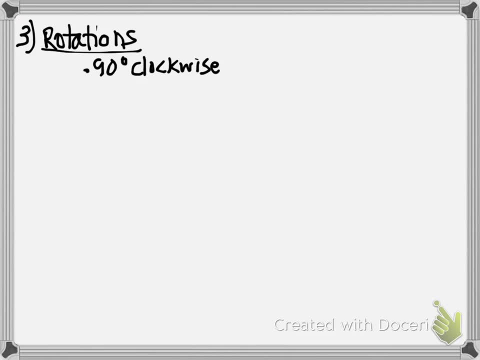 Now that actually does describe. What other rotation would have a second rotation, What other rotation would have the same exact change as the 90 degrees clockwise? Kaleo, It's what adds up to give me the 360. And it's going to be the opposite direction. 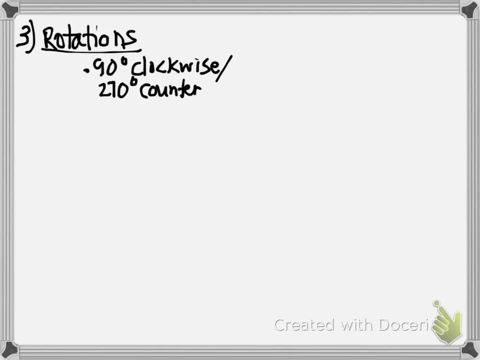 So it would be counterclockwise. Okay. So your x, y And again, if I draw a picture real quickly of this, And we're here and we're going to rotate clockwise- Okay, Notice the sign. that's going to change. 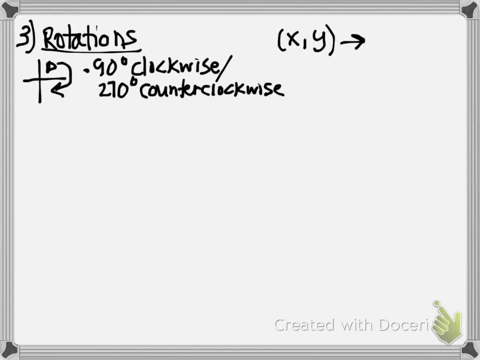 Your y went from being a positive one to a negative one, So we're going to end up changing. Make sure I get this right. Okay, We are going to swap spots with the x and the y And on this one, if we're going 90 degrees clockwise because we're swapping spots, 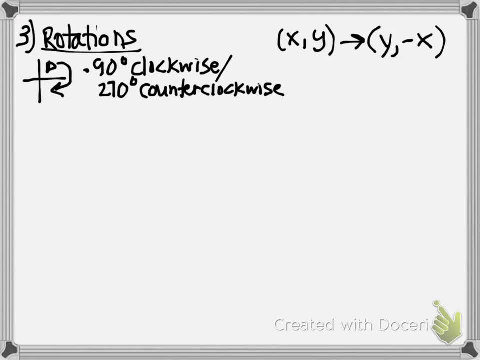 we are going to change the sign of the x. Okay, So when we have that rotation, The x is actually going to have to change its sign. There was an example of homework that you guys did And most of you had the wrong starting point for your triangle when you did your rotation. 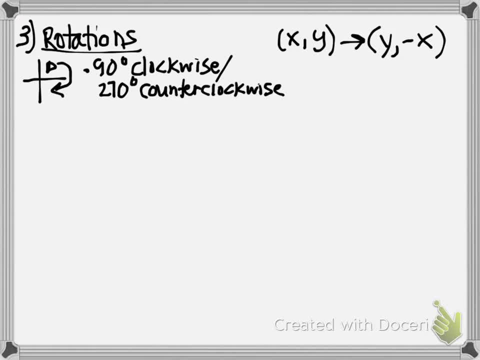 And so, even though it looked good, it actually was wrong Because of not swapping the sign properly. Then we also have a 90 degrees counterclockwise, Which is the same as what other rotation? 270 clockwise, 270 clockwise. 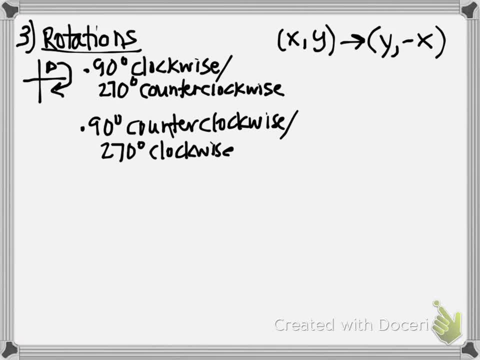 We're not going to whistle in class, Thank you, And you're supposed to be taking notes, not scribbling on the spiral I gave you. We're still going to swap the x and the y, But we're going to make sure that we change the y's value to its negative first. 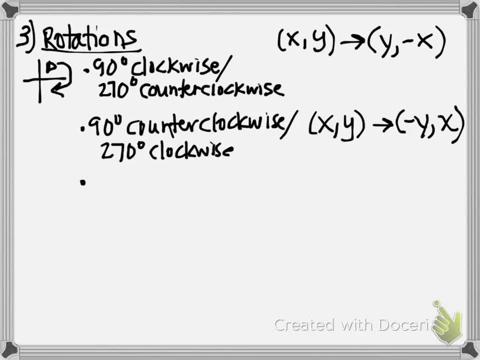 Okay, The last one is the 180. And notice that the 180 does not get a clockwise or counterclockwise, Because we end up in the same exact position both ways. So we just say it's a 180. And what's nice about it is that the x and the y don't swap spots. 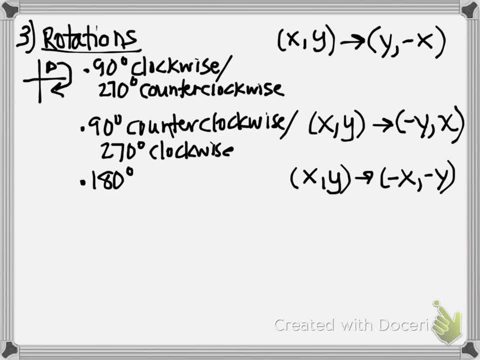 What they do is they change signs. So for me memorizing those three in particular are the most helpful. The others I can logically kind of figure out, But this one it's going to make sense if I deal with the change in my values. 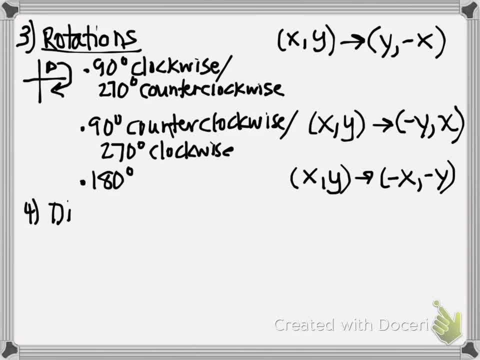 And then the last one is the dilation, And we're going to use k to represent the dilation amount for both of them. But I'm going to give you a specific about what that k is going to look like. So the two different ones. 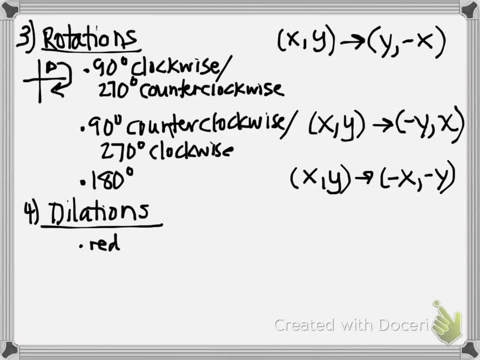 The first one would be a reduction, And when I multiply by this k value, it's going to shrink my original picture. So what numbers did we say I would need to multiply by in order to shrink an original shape? What kind of numbers?